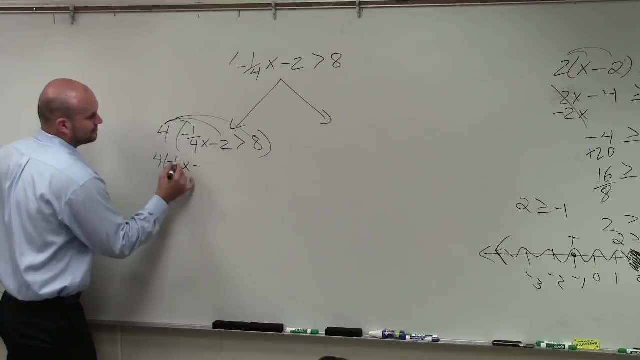 4 times negative. 1 fourth x minus. Where did I lose you? I'm multiplying 4 times every one of these terms. If put that over 1.. 4 over 1 times negative. 4 over 1.. The 4's divide out: 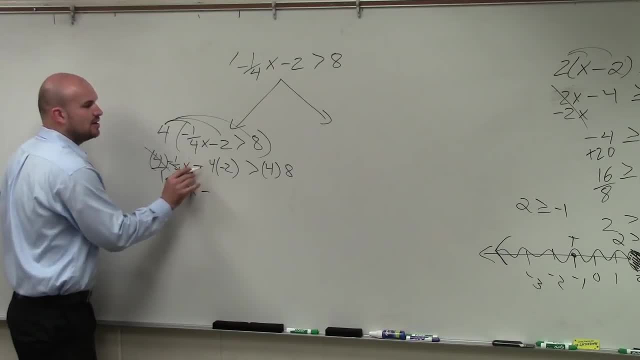 Negative 1 divided by 1 is negative 1x minus negative. 4 times negative, 2 becomes a positive 8 greater than 32.. Can you guys solve this equation now? No, Why not? OK, The next thing you guys can do is if there's only one fraction, 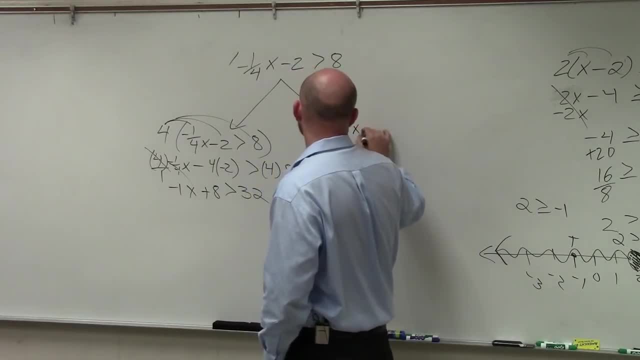 just worry about the fraction when you have to. If I have negative 1 fourth x minus 2, greater than 8, what is the first thing we need to do? anyways? The first thing we need to do is always undo addition and subtraction. 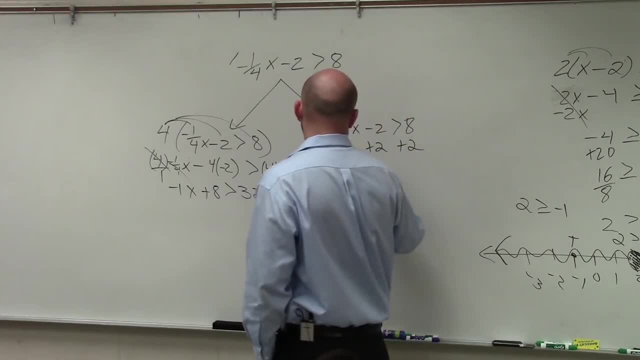 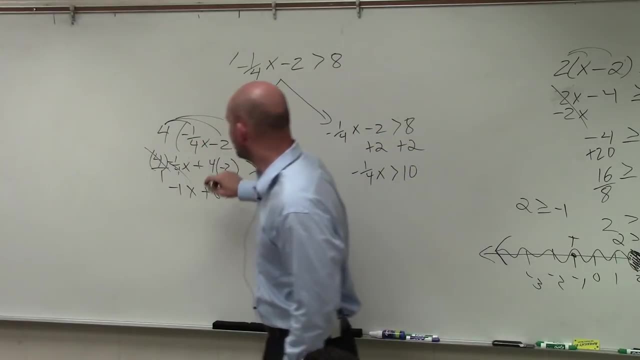 So we don't even need to worry about this fraction right now. Yeah, Negative 1 minus negative 2.. Oh wait, Actually never mind, I did make a mistake there. It's 4 times negative 2, right. 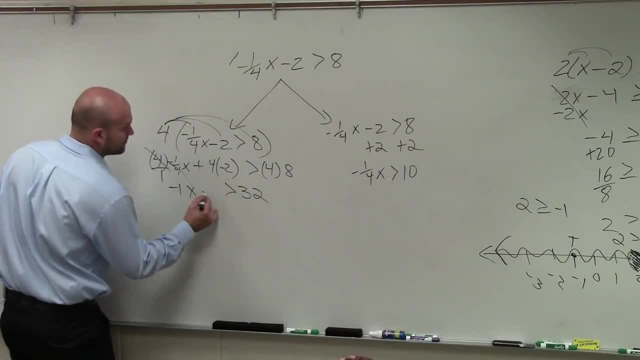 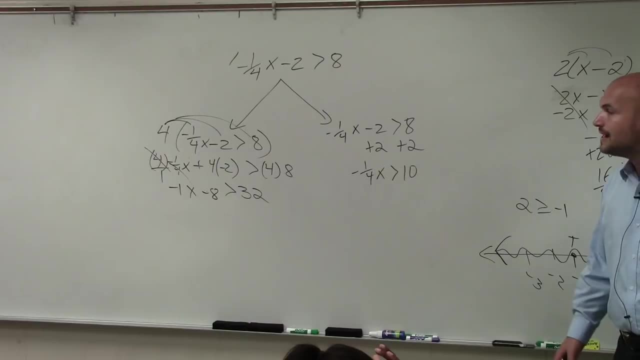 So that should be a positive 4.. Thank you, So now I have two separate equations Here. all I did was add a 2 on both sides. Now how do we get rid of a fraction when it's just a fraction times a number? 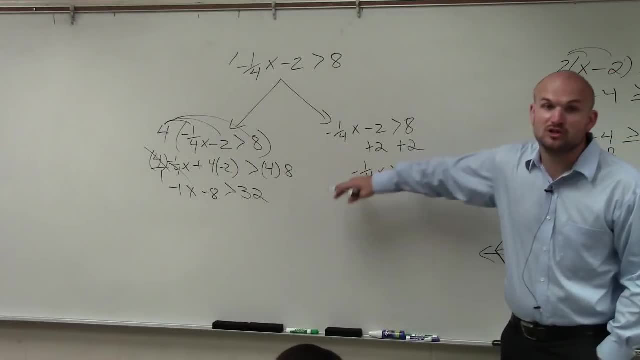 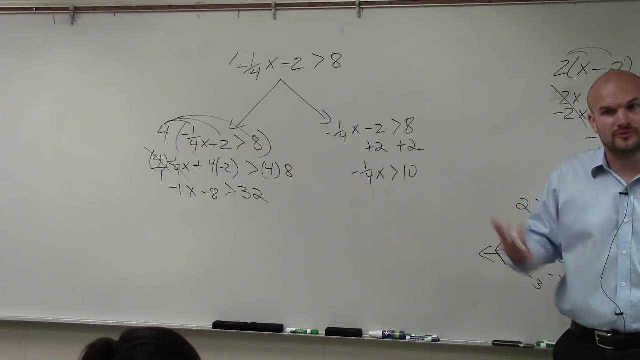 Well, you could divide. Now my variable x is being multiplied by negative 1, fourth. So to undo multiplication of a fraction, we multiply by the reciprocal. So I can multiply by a negative 4 over 1.. I want to multiply. 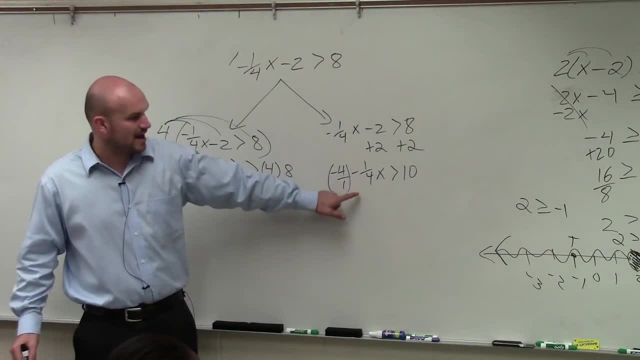 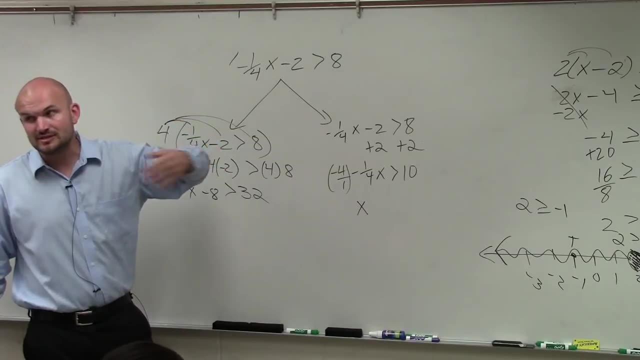 I'm going to multiply by negative 4 over 1, because I want to make this a positive variable. And this is where the reason why, in that problem, I wanted you guys to always solve for the positive is because a lot of students, including myself, 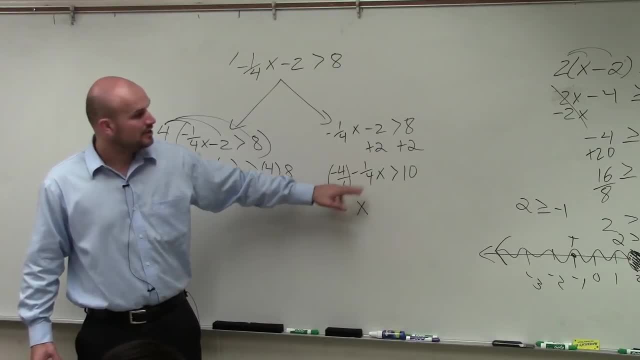 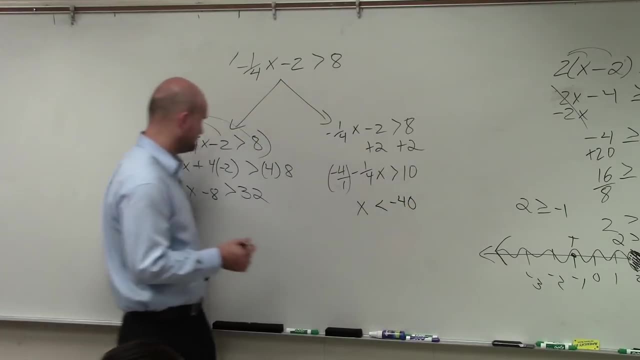 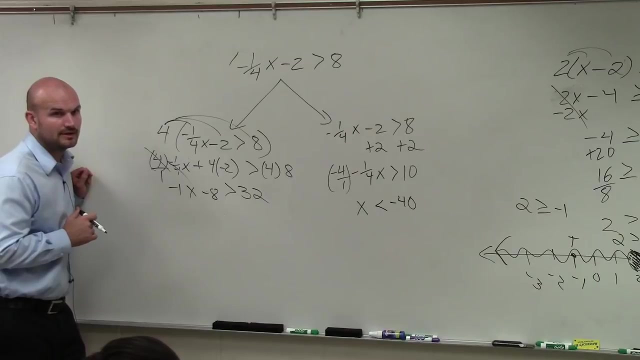 forget, when you multiply or divide by a negative number, you have to flip the inequality symbol, So now this one becomes negative 40. OK, Huh, Do you have? Yeah, Why would I go? Why would I go over it? 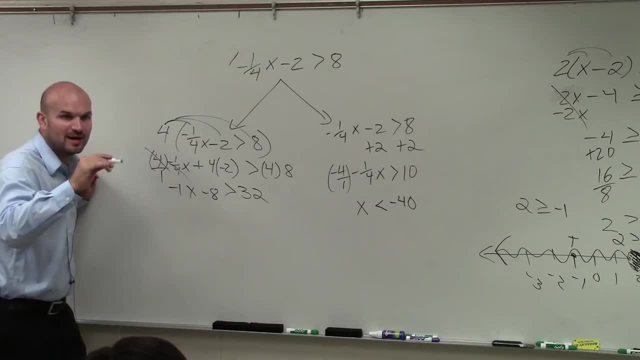 Write it down. Flip the sign when you multiply or divide by a negative number. when you're solving for a variable, Write it down Here. let's go and do this. I add 8.. Negative x is greater than 40.. Divide by negative 1.. 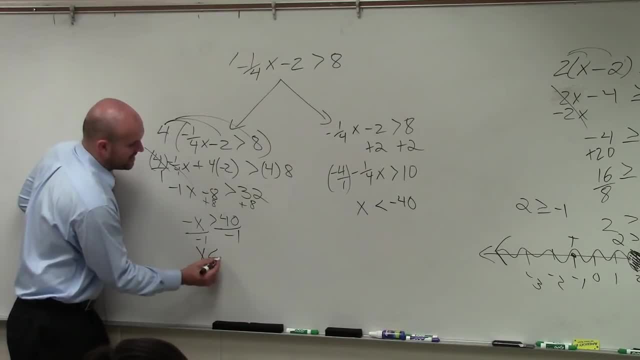 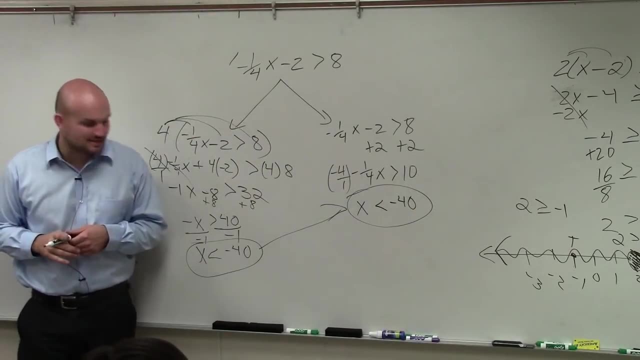 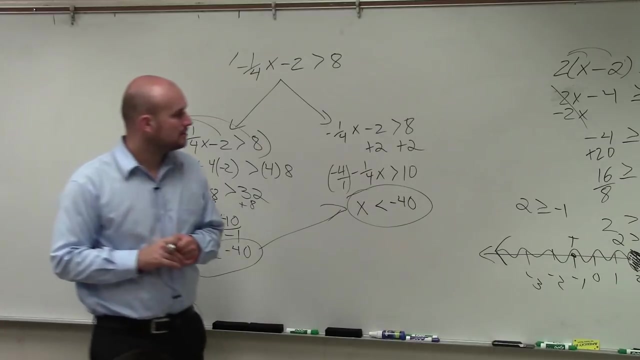 Divide by negative 1, because you have to solve for x. x is less than negative 40.. Notice, ladies and gentlemen, I solved it two different ways And I still get the same answer. So now we've got to go and graph our solution. 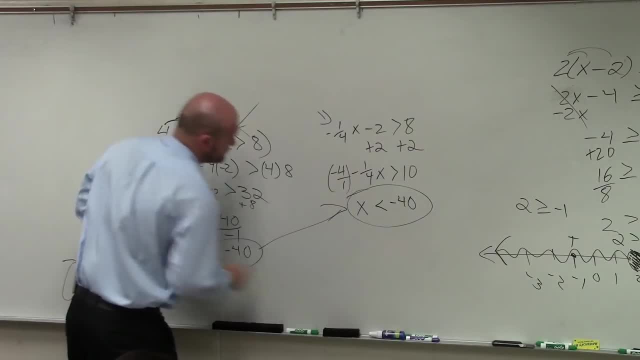 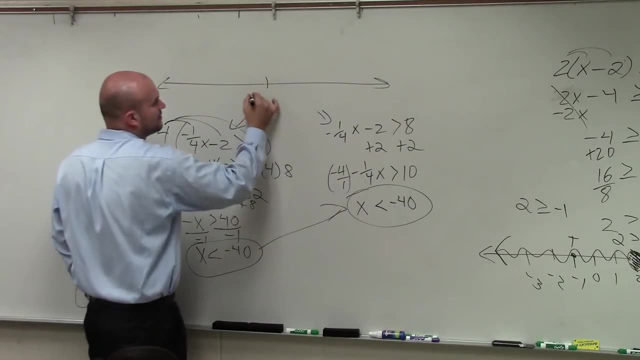 So again, just like I was going back, I'm going to leave that. I'll just erase the problem. So now to graph the solution. what I tell you guys to do is go ahead and find negative 40 and then do larger numbers. 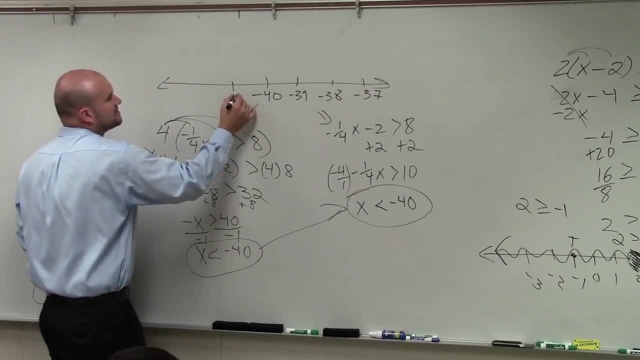 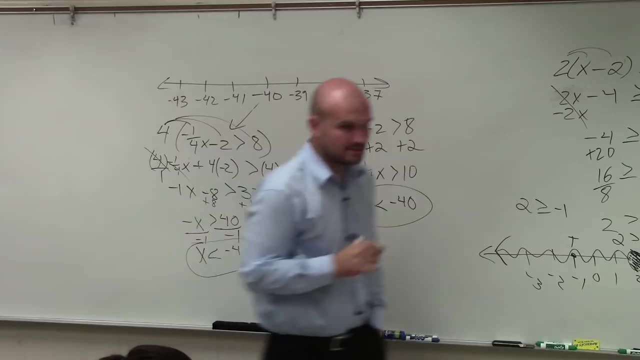 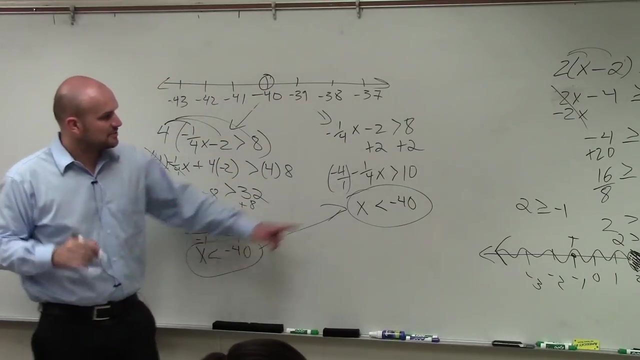 to the right And the smaller numbers to the left, And you will have to create your own number lines. So now we get into this and we make a dot at negative 40. And, per our discussion in the last class period, is that open or is it closed? 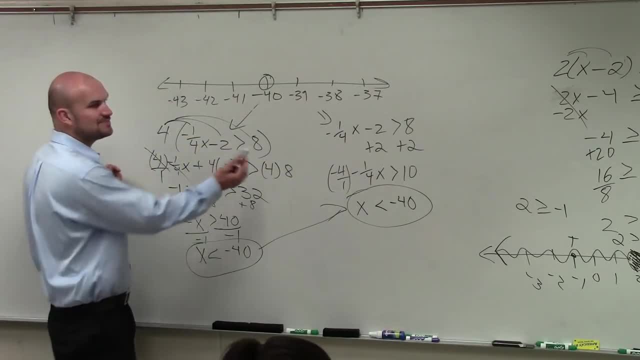 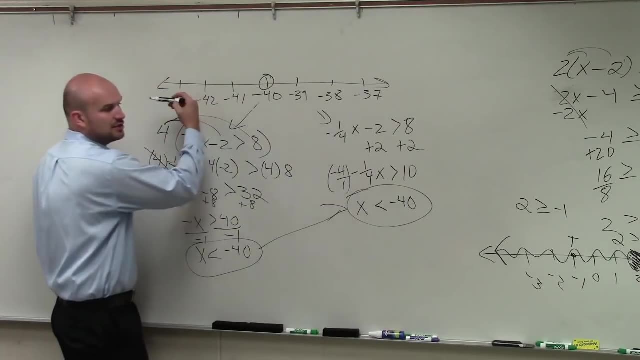 It's open because it's not true, And then you can do test points if you like, But since my variable's to the left of my inequality symbol, you can see one: the inequality symbol is telling us to go to the left. 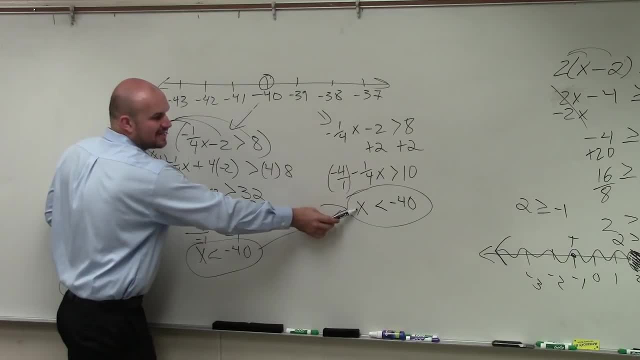 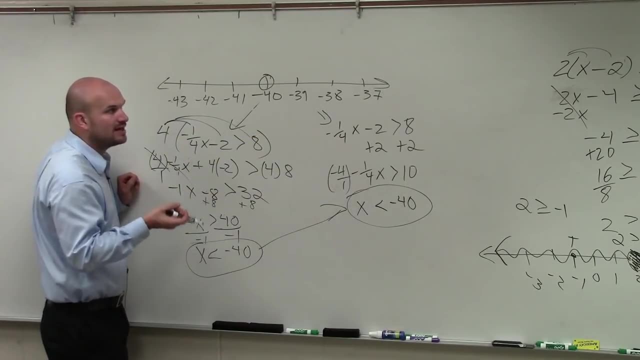 And let's just say it out loud. OK, Let's just say it out loud. What numbers x is less than negative? 40?? Is that numbers to the left or to the right? Left, Yeah, Think about negative again as owing money. 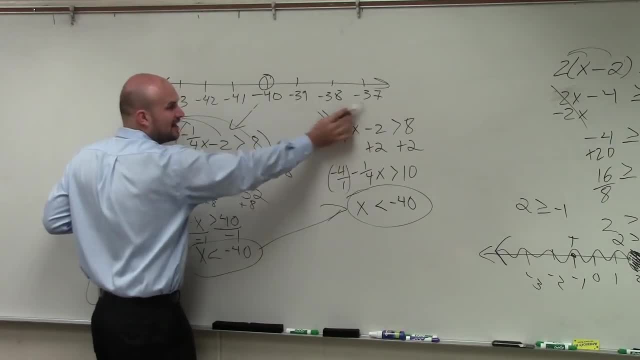 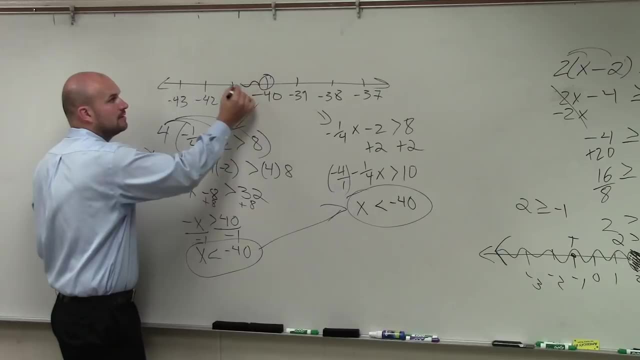 If you owe $43 compared to owing $37, do you owe less money? the more negative it is? Do you have less money, the more money you owe. Yeah, Yeah, So it goes to the left. OK, So you guys lost five minutes. Second period lost 10 minutes. OK, All right.